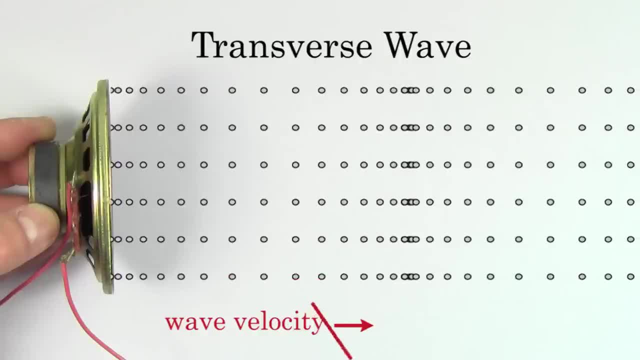 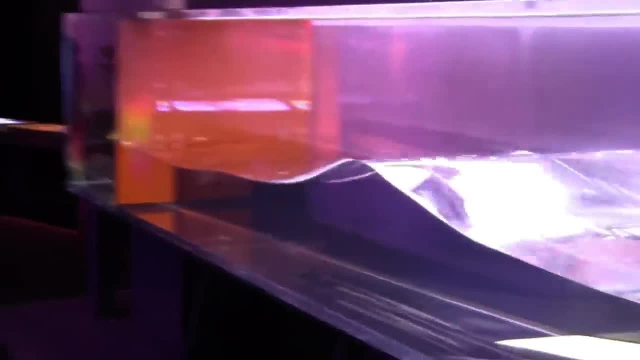 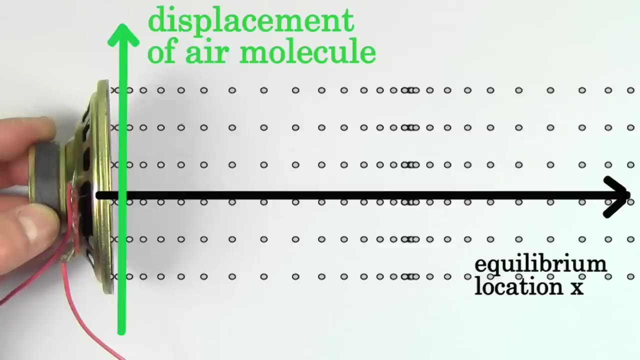 The other type of wave is called a longitudinal wave. Transverse waves happen when the wave velocity points perpendicular to the oscillations of the medium. Waves on a string or waves on the surface of water are examples of transverse waves. If we look at a graph of the air displacement versus position of the air, we can see that as the wave travels, the shape of this wave travels to the right. 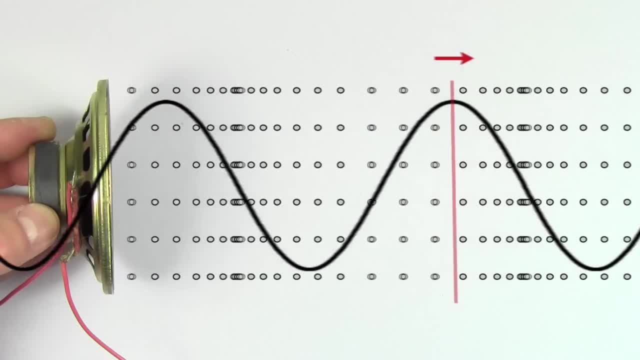 So the speed of a sound wave can be found by finding the speed of the peaks or the speed of the valleys, or the speed of any single point on the wave shape. To figure out the speed of a sound wave we can use the speed of the peaks or the speed of the valleys, or the speed of any single point on the wave shape. 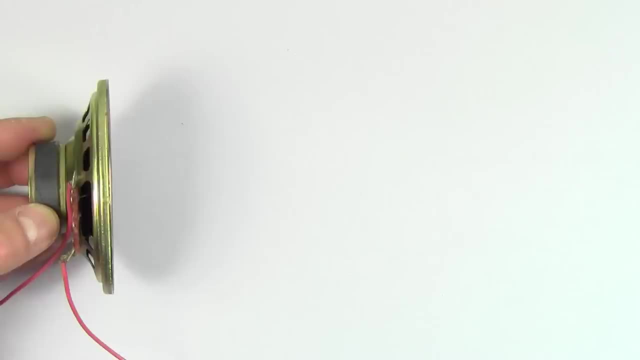 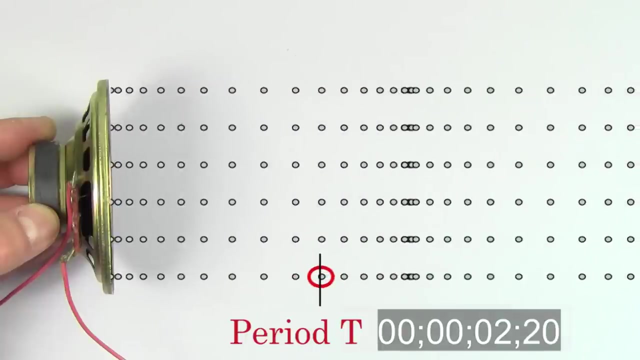 to build out a formula for the velocity of a sound wave. Let's look closely at what's happening here. Watch one of the air molecules. It takes one period for this molecule to move back and forth through a full cycle. During this time, the wave shape has moved forward one complete wavelength. 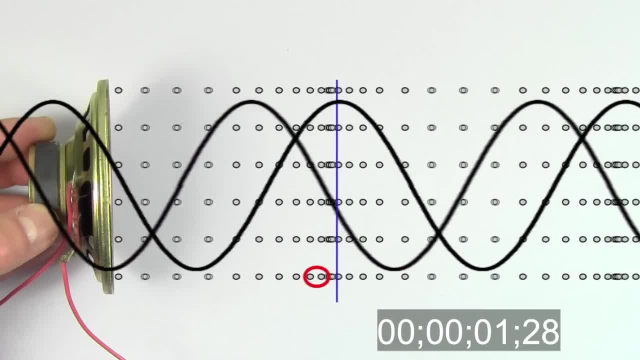 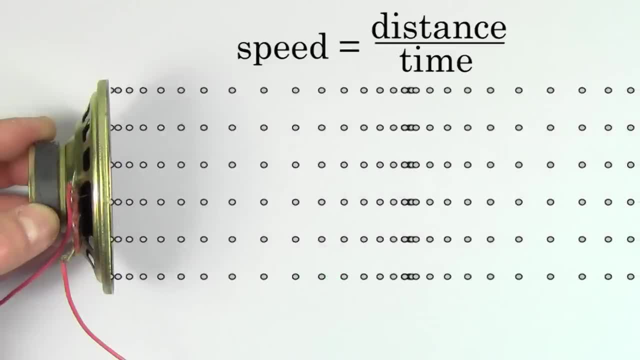 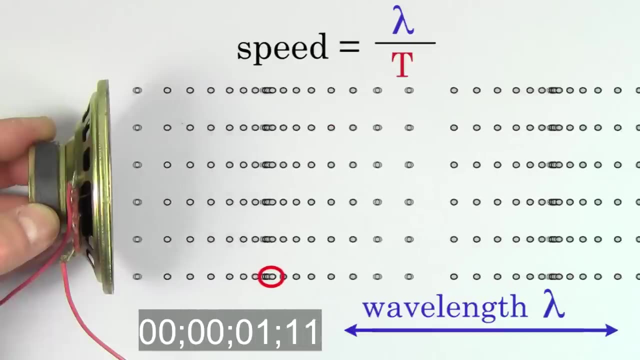 This is because the wave has to overlap with its initial shape after one period. Now, since speed is defined as the distance per time, The speed of a sound wave has to be the wavelength of the wave divided by the period of the wave, since the wave is traveling forwards one wavelength per period. 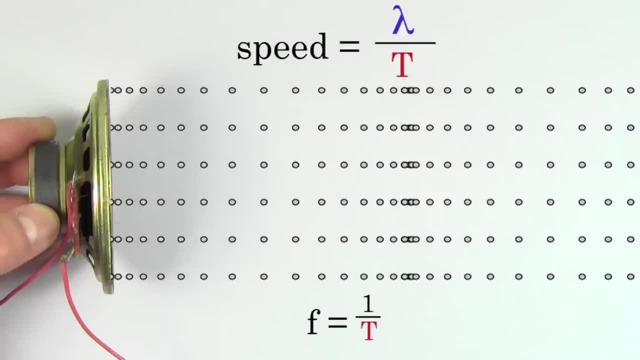 Or, since the frequency is defined to be 1 over the period, we can rewrite this formula as: speed equals wavelength times frequency. This formula is accurate for all kinds of waves, not just sound waves, because a wave has to move one wavelength for every period. 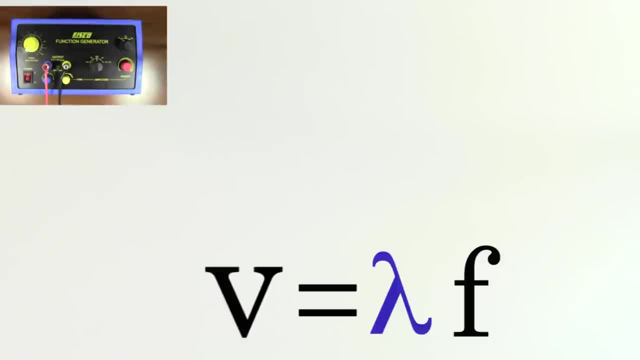 Be careful When looking at this equation. you might think that if you adjust the setting on your speaker and increase the frequency, you'd also be increasing the speed of the sound wave, But that's not what happens. If you increase the frequency, the wavelength will decrease by that same factor. 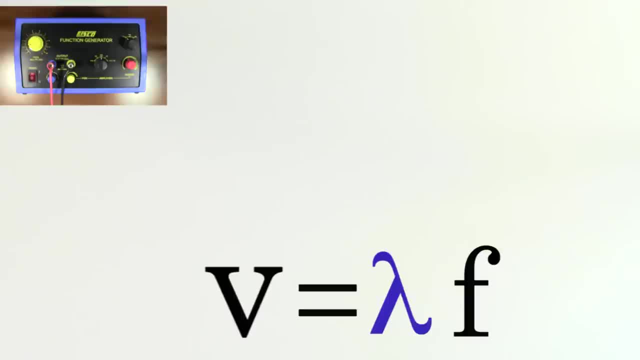 and the speed of the sound wave will remain the same. In fact, there's nothing you can do to the speaker that would increase the speed of sound. So how can we change the speed of sound? Well, the only way to change the speed of sound 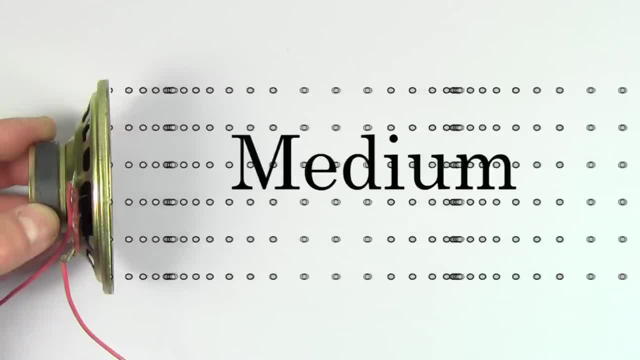 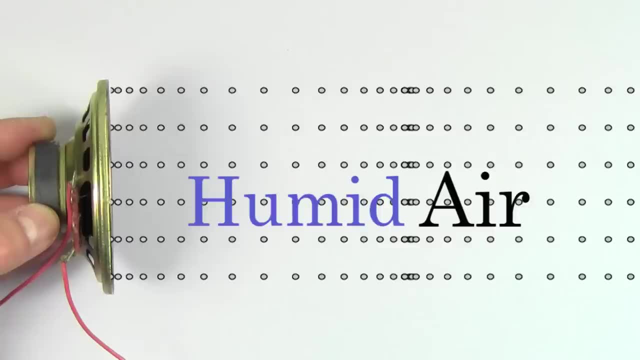 is to change the medium or the properties of the medium that the sound wave is traveling in, So to change the speed of sound. in air you can change things like the temperature of the air or the humidity of the air or the density of the air.